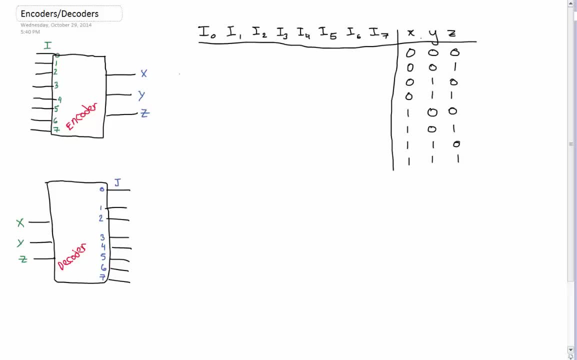 So this is the truth table for an encoder. It's kind of similar to a multiplexer in that we're still dealing with cases or conditions. So when x, y and z are equal, we're going to have 8 outputs and Zed. oh crap, I'm still getting used to one note. I have no idea what's. 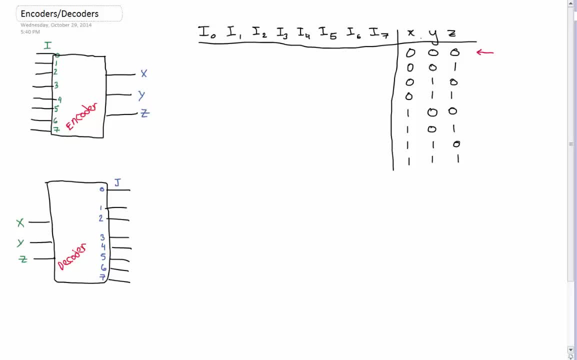 happening half the time when X, Y & Zed are all zero. that means that our input will be our very first input, just because this is the first kind of condition of X, Y & Zed. so that will be one and we're just going to iterate all. 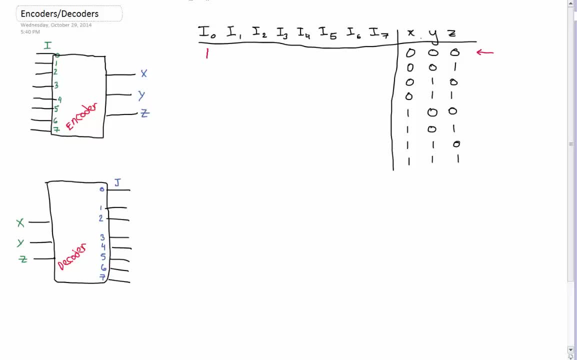 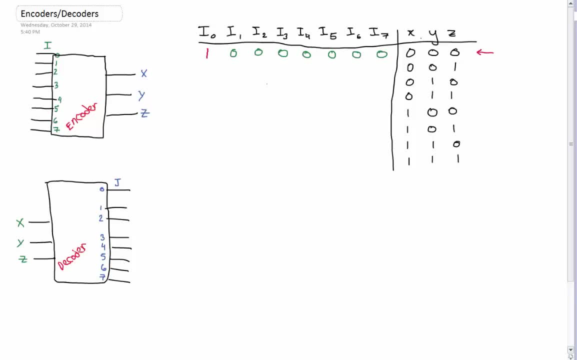 you're only going to have one, one value on each row of inputs for the encoder. alright, so now we're on our second condition. so another way of saying it is that if the input is I1, so if you have I1 as equal to 1, then x, y and z will be 0,, 0,, 1.. 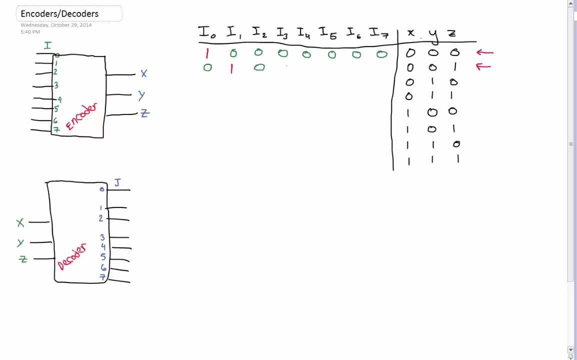 So we'll do our zeros now Because, remember, we can only have one value per row of inputs And we're just iterating down. Honestly, we're just going down the list. So now i1 is 0, because we're on the third. 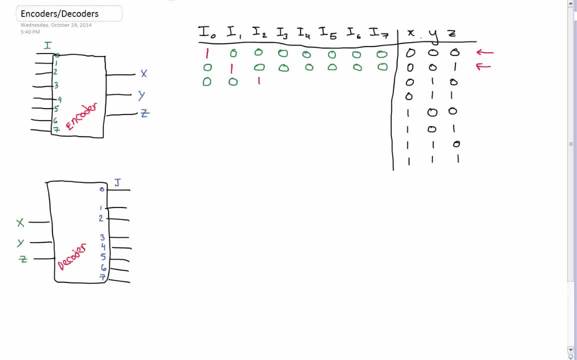 row now. Okay so I think you guys get the idea, So I'm going to cut out and fill out the rest of the table. Okay, so this is our completed truth table for an encoder And, as you can see, we have kind of this diagonal. 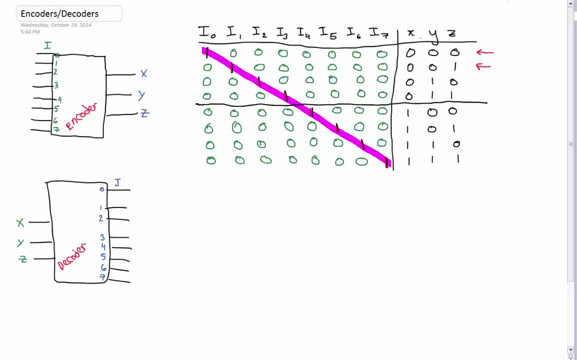 thing here. I'll just retrace the one so we can see them better. So again, we're just kind of going down the list here. So we have input 0 here, which is our very first input at the top right here, And when that is 1,. 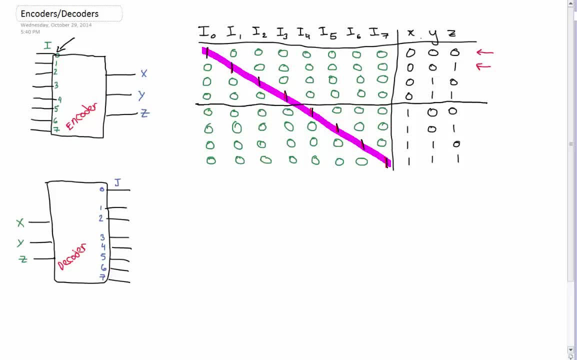 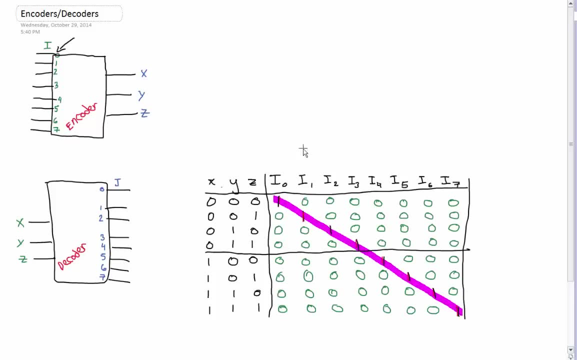 then we'll have 0,, 0, 0 for x, y, z, And then we just kind of go down the truth table. So now we're going to look at decoders. Okay, so decoders are really just the opposite of encoders. So I took the truth. 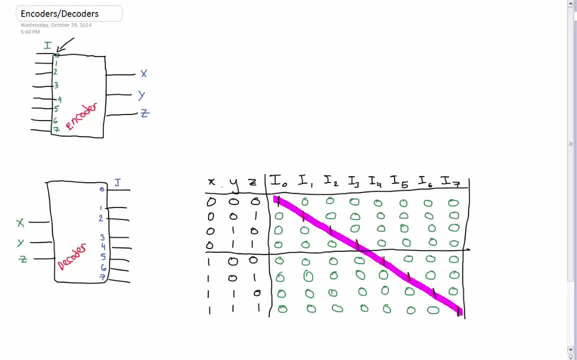 table from the encoder. that we just did And I just reversed it And it's honestly, it's the same concept. So I'm just trying to change the cursor here so I can follow it a bit better. So when we have, x is 0,, y is 0,. 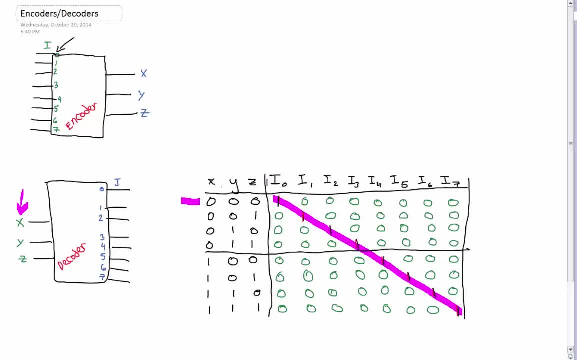 and z is 0, which is this condition here, our first condition. then i0 will be 1.. And again we can only have one 1 value per row of outputs here instead of inputs. So it's the same thing. We're just really looking at the x, y, z. So when x, y and z 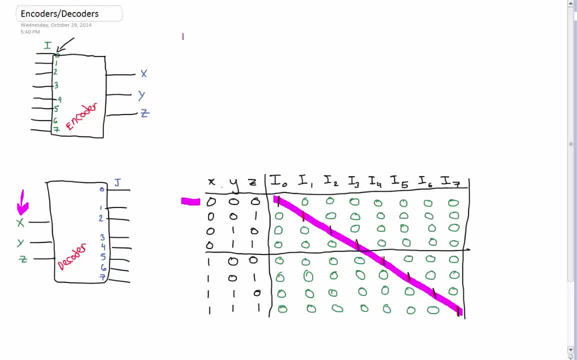 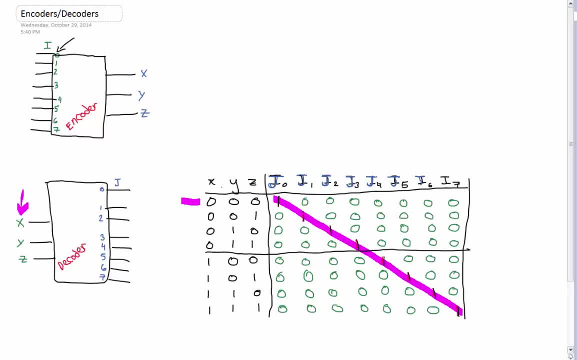 I wanted to differ the encoder input from the decoder output. So those are all j values. So when x, y and z are all 0s, then our first output will go out. When x, y and z are 0s, they're 1.. Our second output will go out. 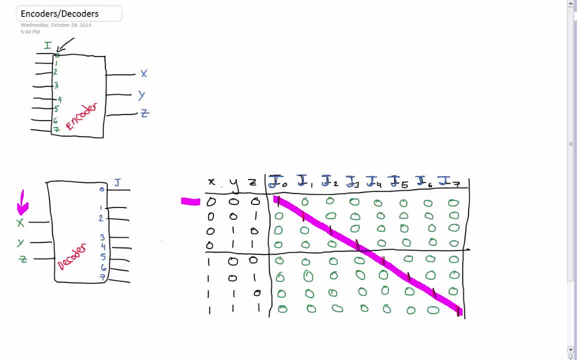 will go out. it's just based on conditions. so again, we're just iterating down the list here. so we go from where's my cursor? there it is. so we go from one- our first condition- to our second, to our third, to our fourth, to our fifth, to our sixth, to our seventh, to our eighth, and we're just. 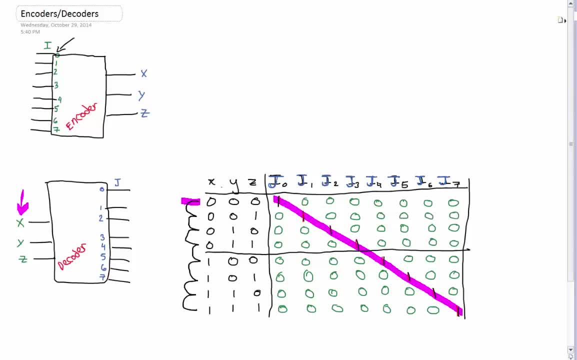 following the diagonal once again. so i hope that was helpful. that's pretty much it for encoders and decoders. feel free to suggest ideas for other videos in the comments section or to ask questions in the comments section. so thanks for watching and